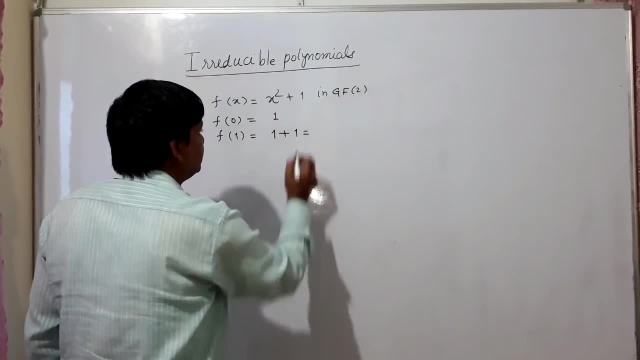 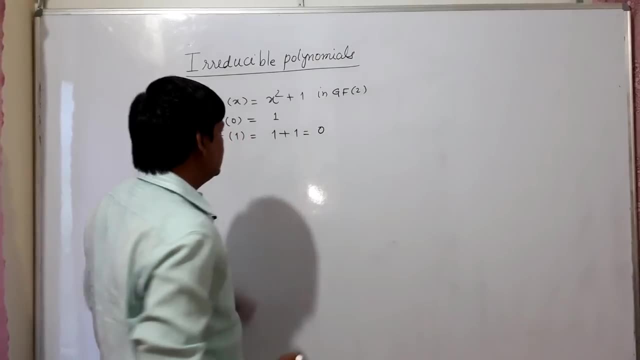 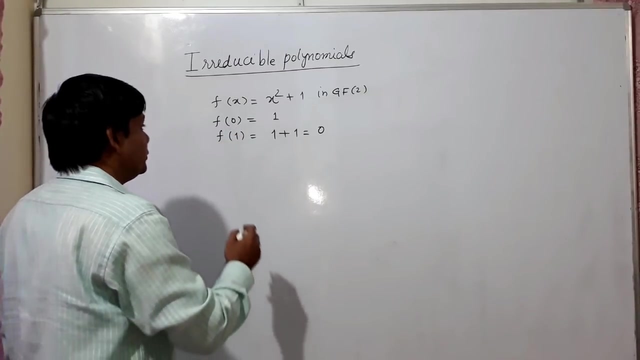 1 into 1 is 1.. 1 plus 1. Field is 2. gf2.. 1 plus 1 is 2.. 2 more 2 will be 0. So its factor is there, which is satisfying x equal to 1.. x equal to 1 means 1 is its root. So. 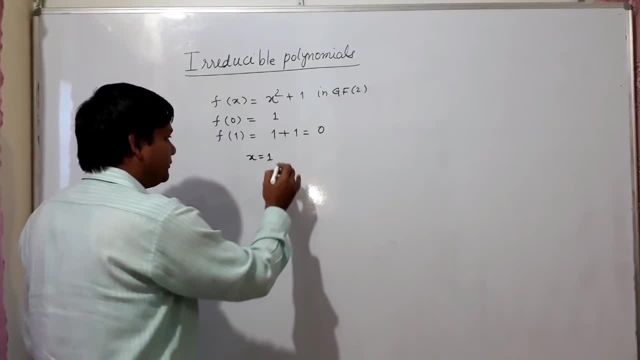 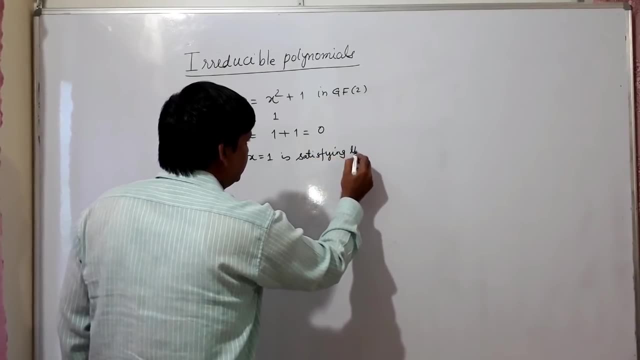 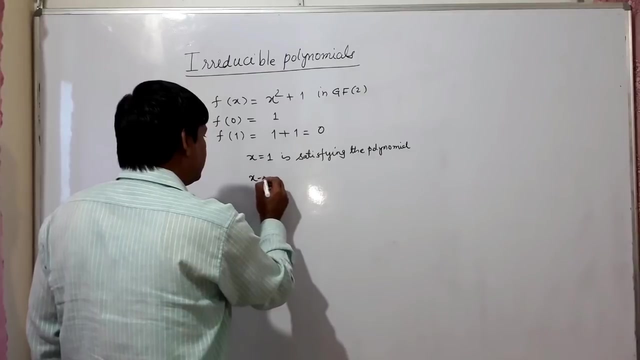 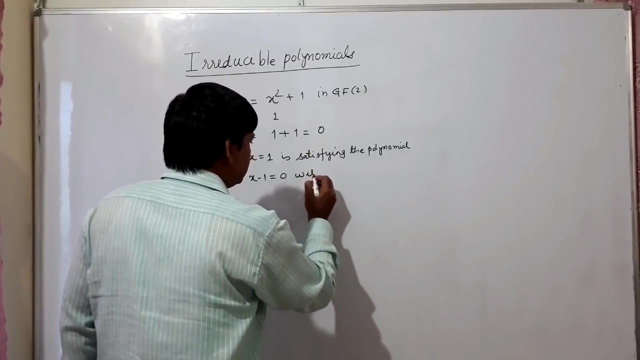 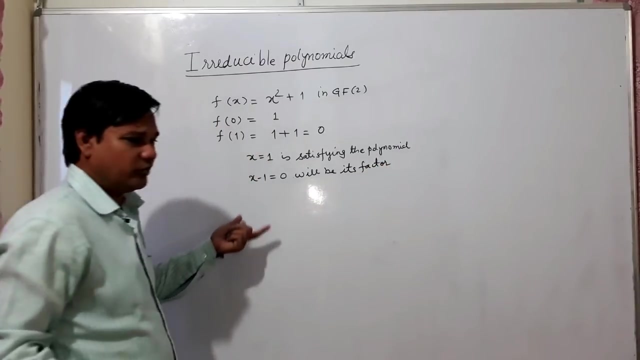 x is equal to 1 is satisfying the equation, It is satisfying the polynomial. It means x minus 1, equal to 0, will be its factor And we know no negative sign is there. It is additive inverse factor. So x minus 1 is 0.. So x equal. 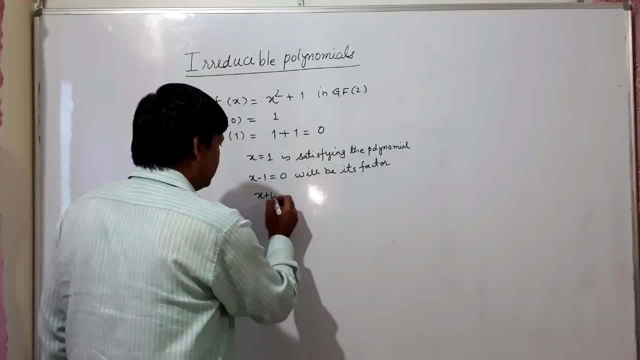 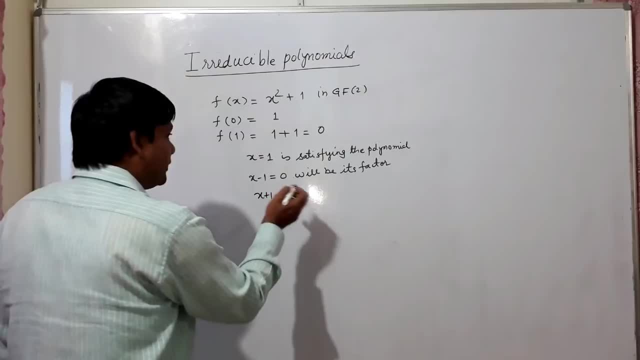 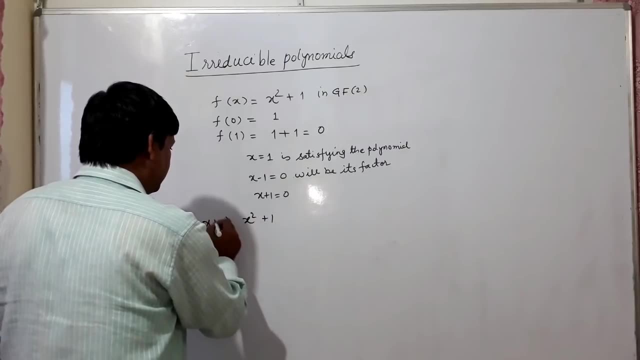 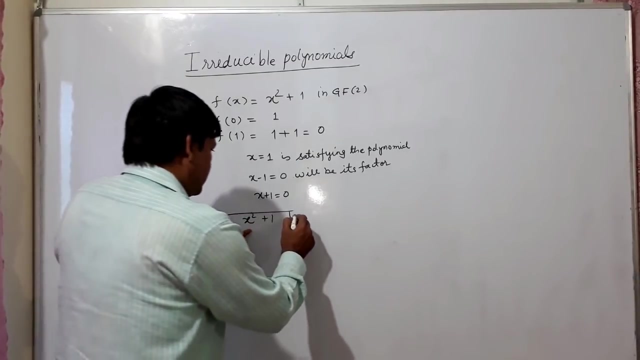 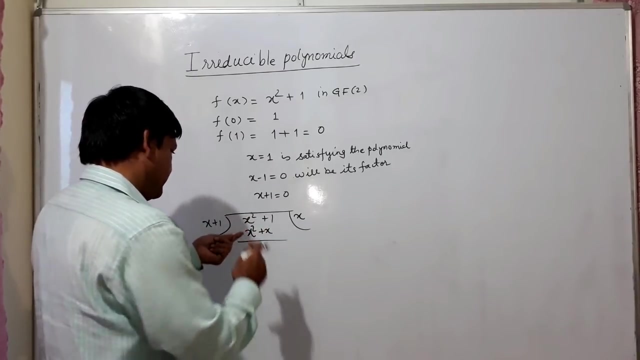 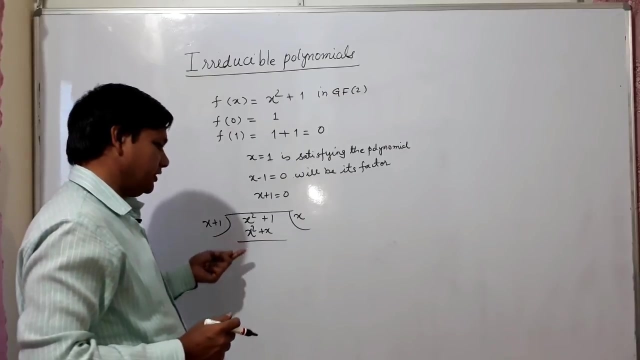 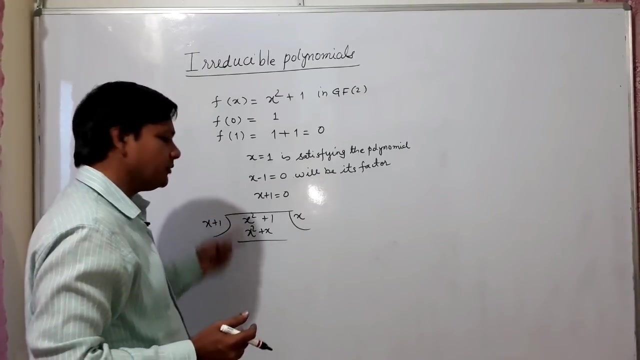 factor. I will check what will be the other factor. If I divide x squared plus 1 by x plus 1, x into x, it should be x here, x squared plus x. we shall have to divide x, Subtract it x square minus. x square minus means we can check here that will be the additive inverse. no problem, that will be plus. plus will be here. if I add it x square plus x square, it will come out to 0, x is here. 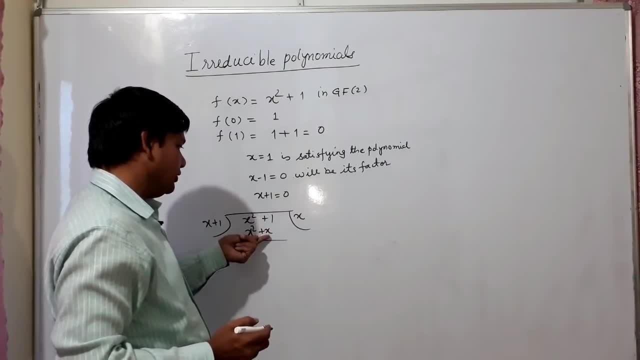 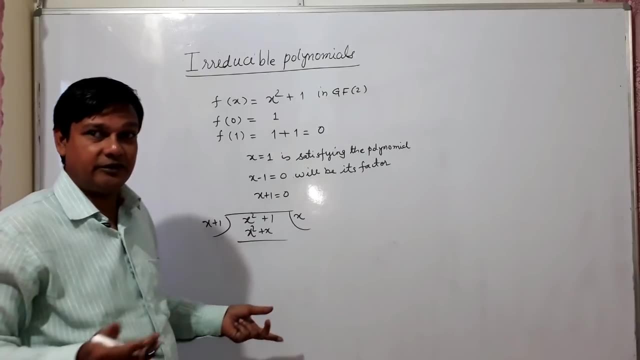 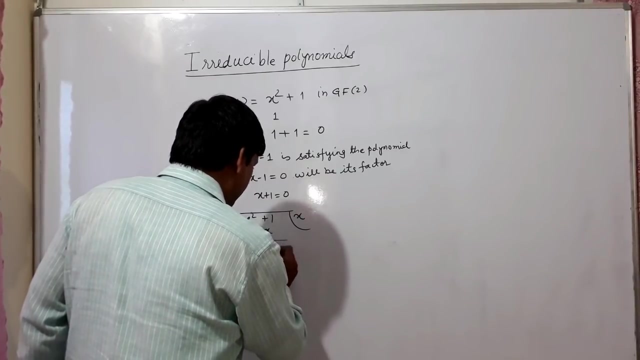 Here subtraction means negative value. negative means I mean its coefficient will be minus 1, minus 1's additive inverse will be x. minus 1's additive inverse will be 1, so this value comes out to be x and 1 was already there, so this will be x plus 1.. 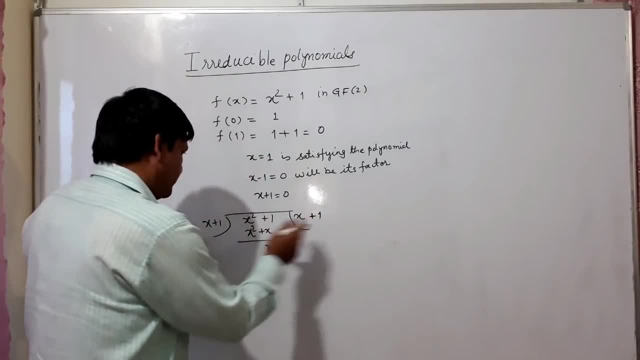 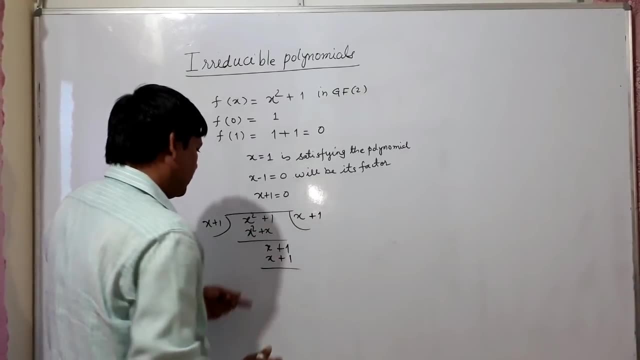 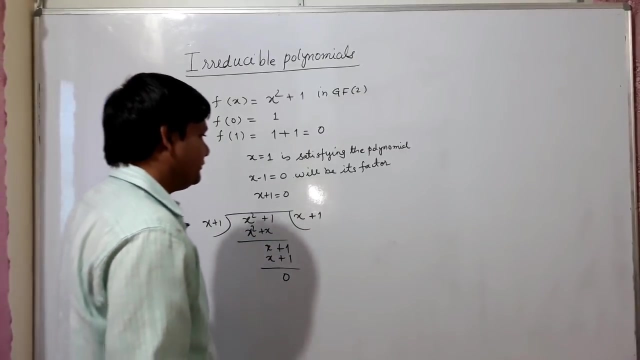 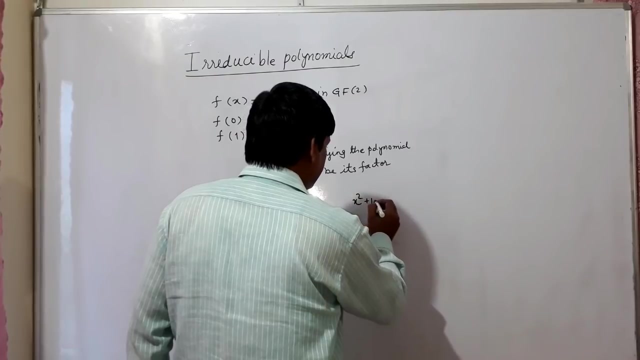 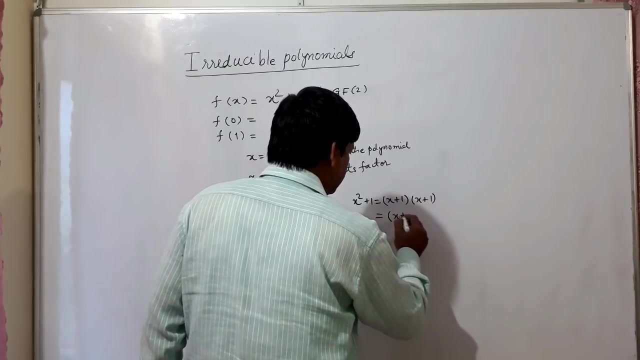 Now I can see: if I multiply it by 1, it will be x plus 1.. If I solve it, it will come out to 0, it means x plus 1 into x plus 1 will be satisfied by this equation. so x square plus 1 is equal to x plus 1 into x plus 1, which is equal to x plus 1 whole square. 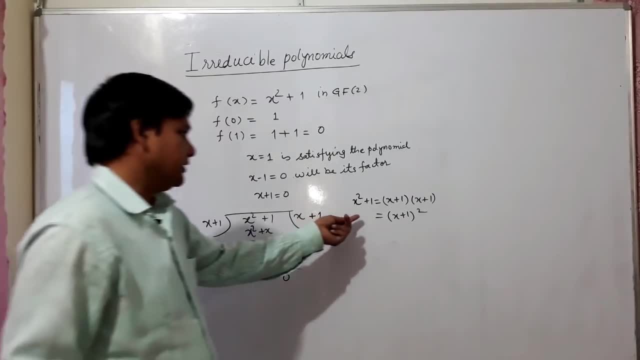 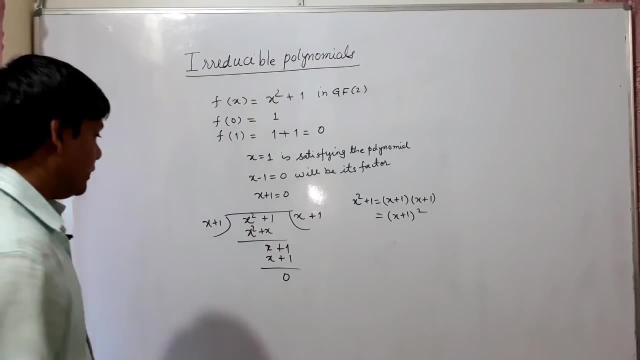 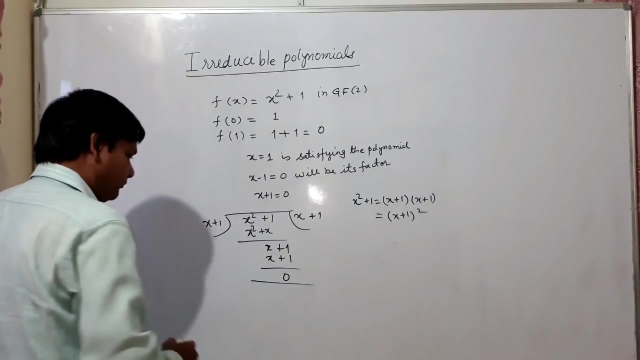 This is x. These are the factors of x plus 1, for x square plus 1.. Now I want to check some polynomials of degree 1, their theories are irreducible or not? Now polynomials of degree 1.. 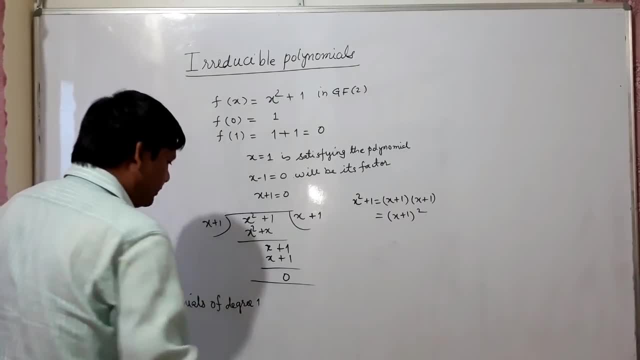 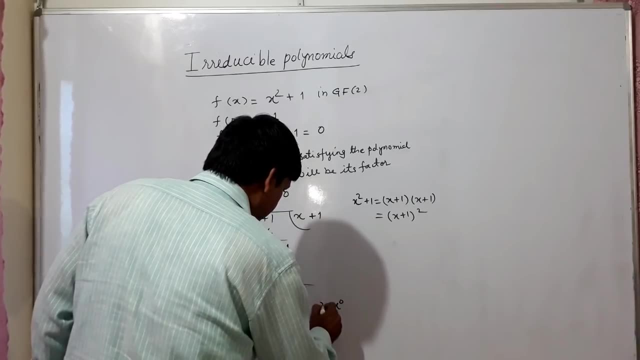 If I see polynomials of degree 1, I can put here x to the power 0,, x to the power 1.. This is fixed. it means its coefficient will always be 1, it cannot be 0.. 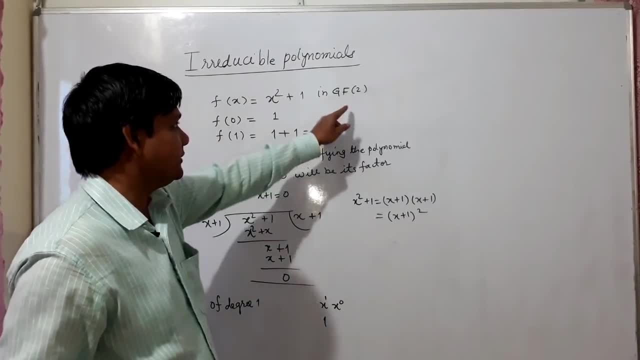 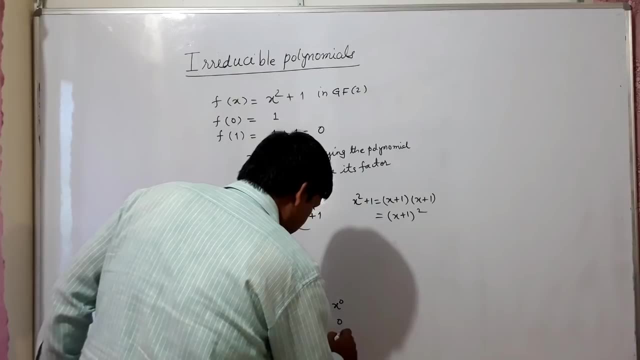 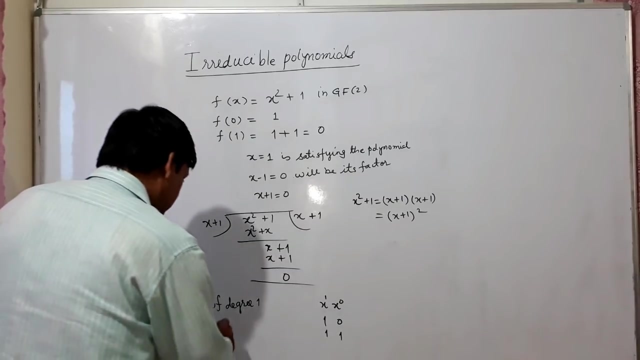 This has two choices, because we are in GF2, so it can be either 0 or 1,, 0 or 1, it will be 1 only. So there will be two polynomials of degree 1, those are: one is x and the other is x plus 1.. 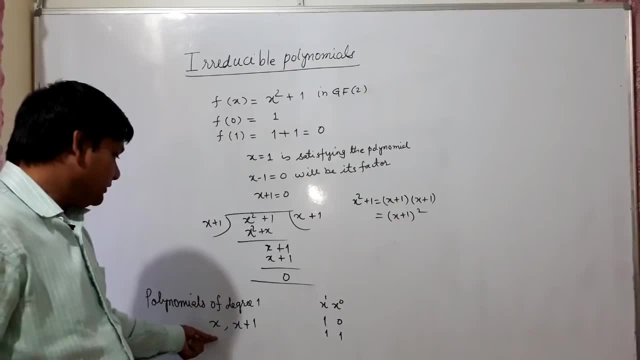 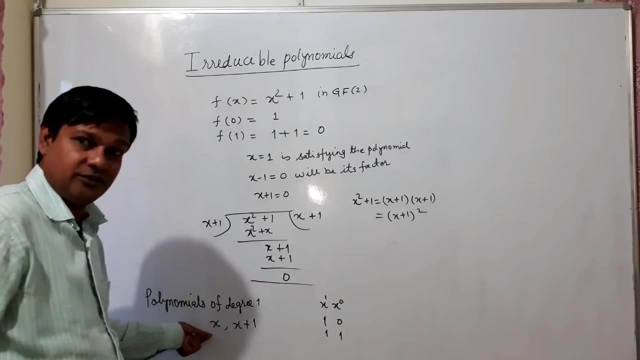 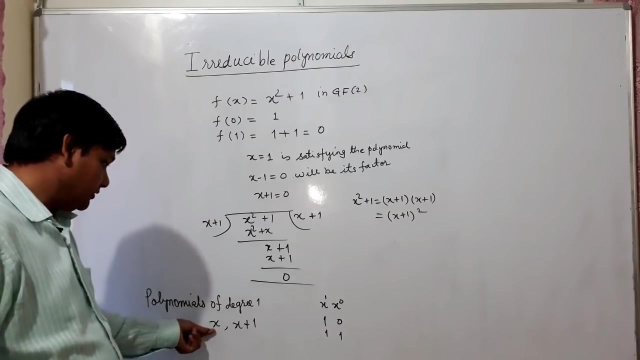 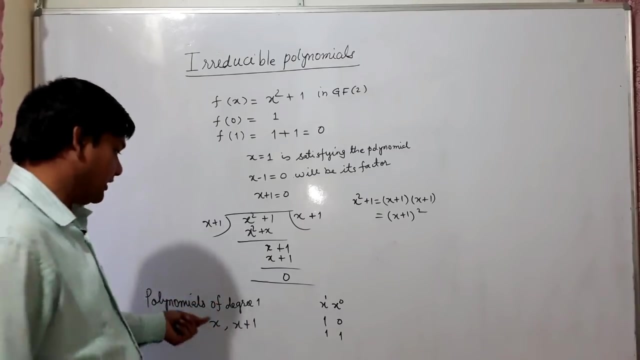 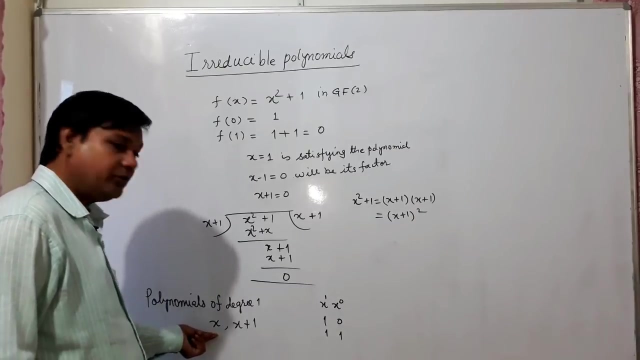 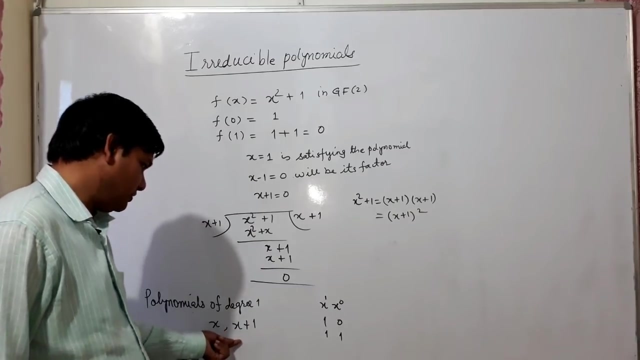 We can see these polynomials cannot be factorized because no x term is there. We can see here: this is x, which cannot be further factorized because its degree is 1.. And we shall have whole degree. it can be 1,, 2,, 3,, 4, or anything else, but it cannot be in fractions, so this cannot be factorized. and we can see x plus 1, this can also be not factorized. 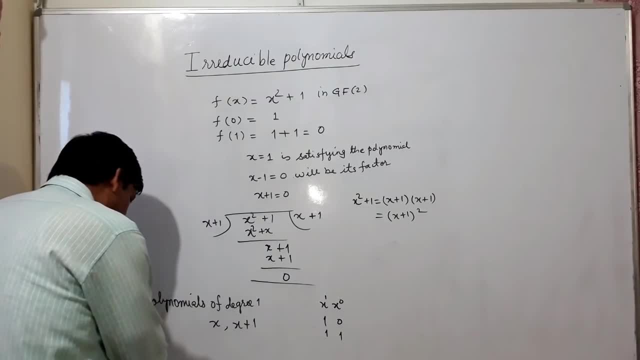 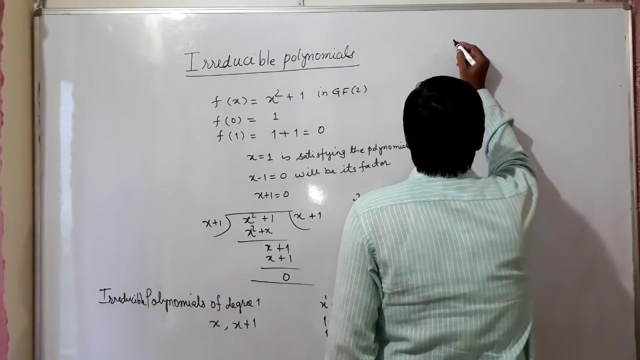 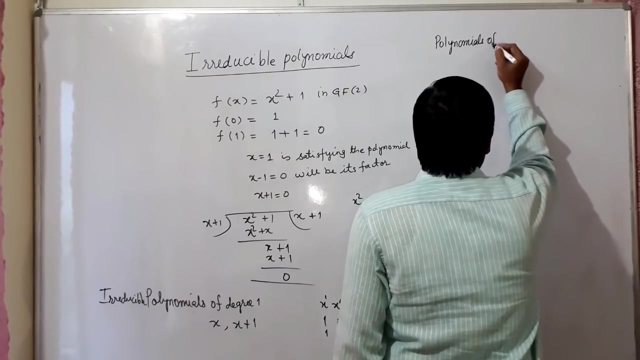 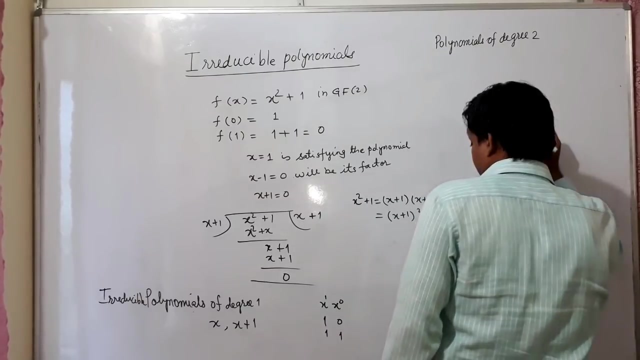 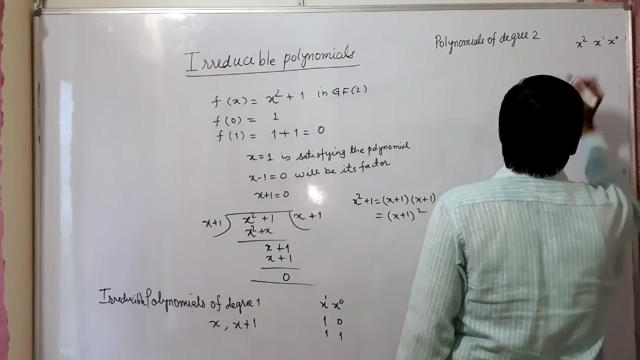 So these are the irreducible polynomials of degree 1.. Now we shall check here polynomials of degree 2, what can those be? x to the power 0, x to the power 1, x to the power 2, this is fixed. 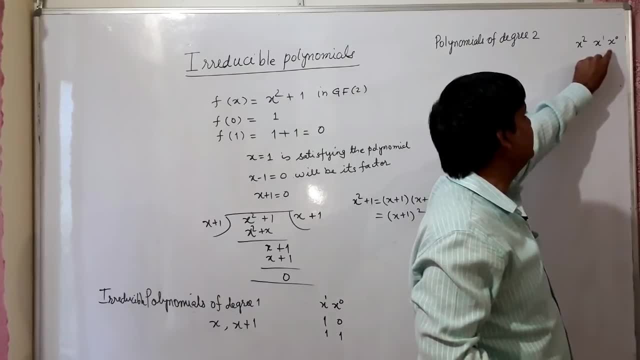 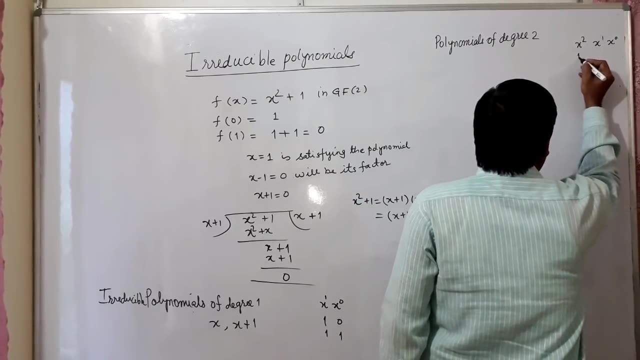 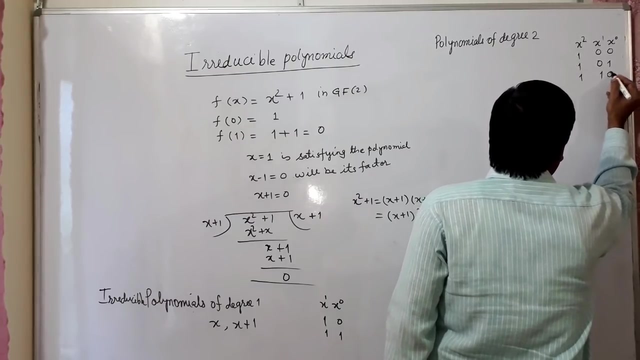 These values. this can be filled in two ways. this can also be filled in two ways, so 2 into 2, 4 ways are there, so it will. its coefficient will always be 1, 0, 0, 1, 0, 1, 1, 1, 0, 1, 1, 1.. 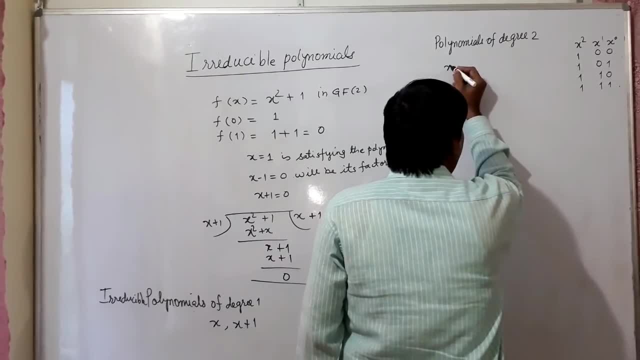 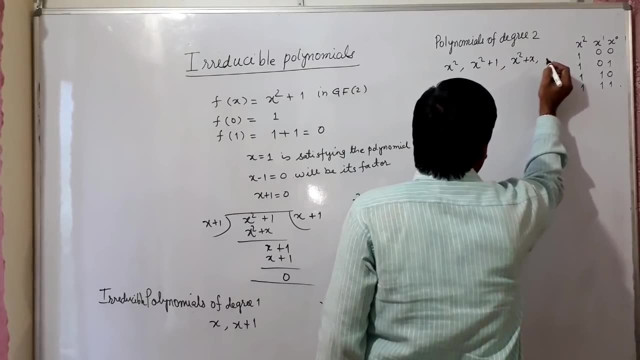 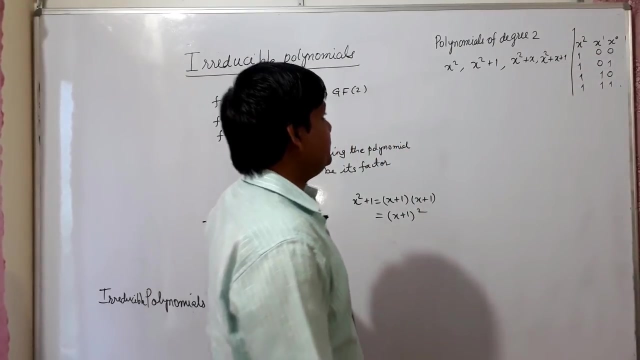 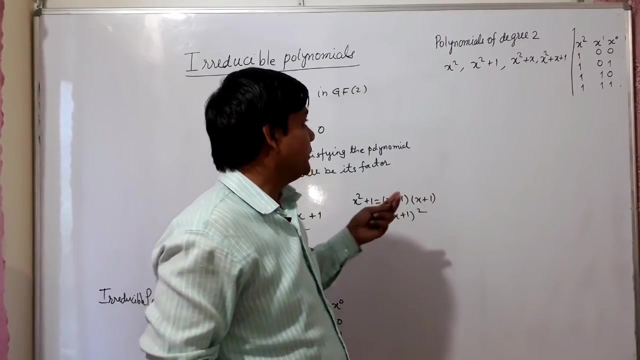 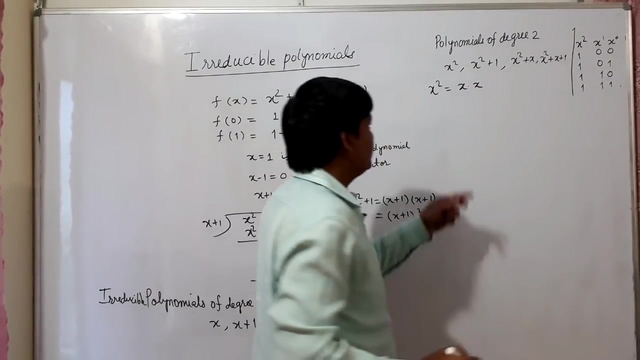 Now polynomials of degree 2 are: one is x squared, other is x squared plus 1.. x squared plus x and another is x squared plus x plus 1.. So we can easily see here: x squared can be factorized in x into x, x squared can be written as x into x, so this is not irreducible polynomial, and x squared plus 1.. 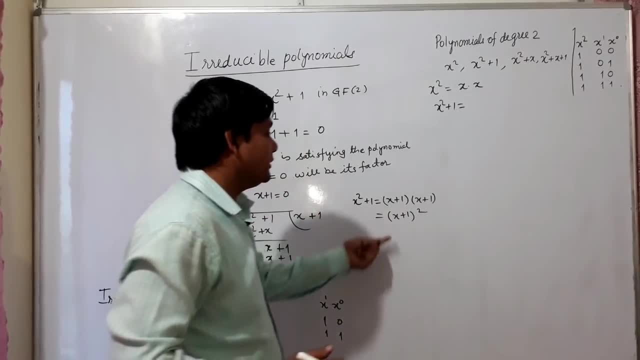 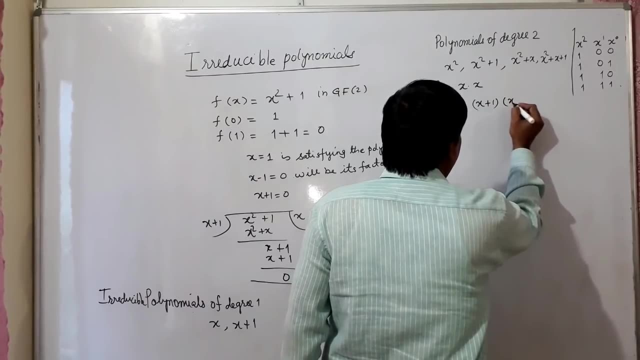 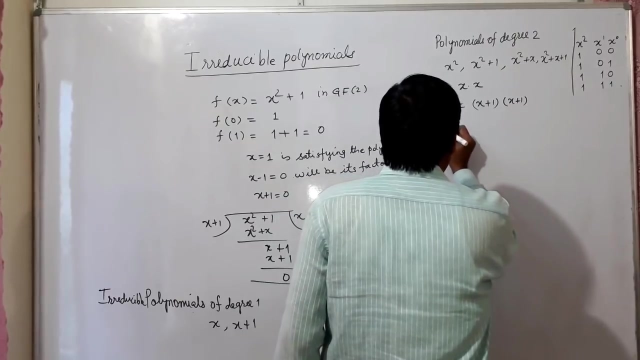 We have already seen here, x squared plus 1 is written as x plus 1 into x plus 1, or x plus 1 whole square. So this is also reducible and x squared plus x can be written as x into x plus 1.. 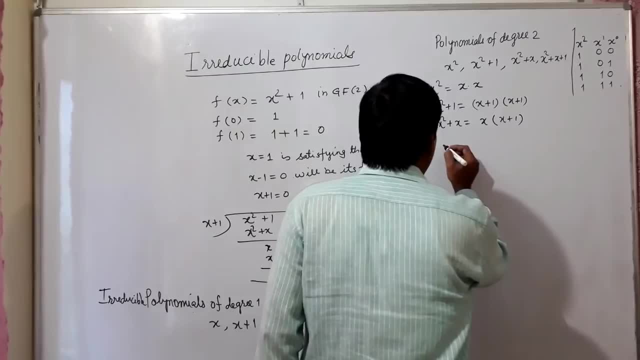 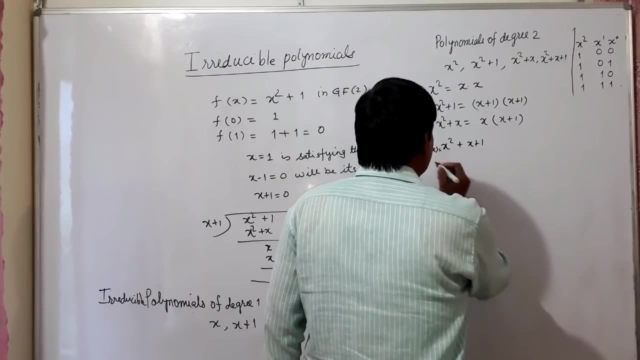 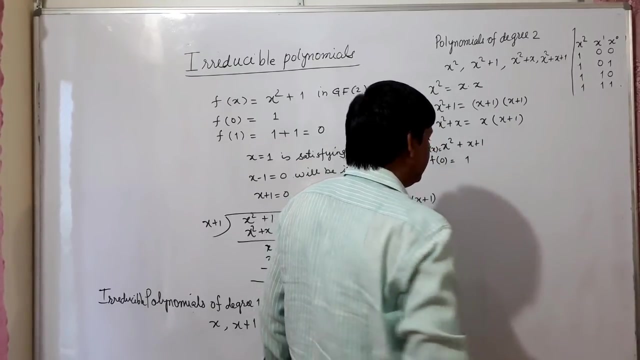 So this is reducible, and I am checking x squared plus x. If I take it as a fx, if I put 0 for x, I will get 0 plus 0 plus 1, this will be 1.. 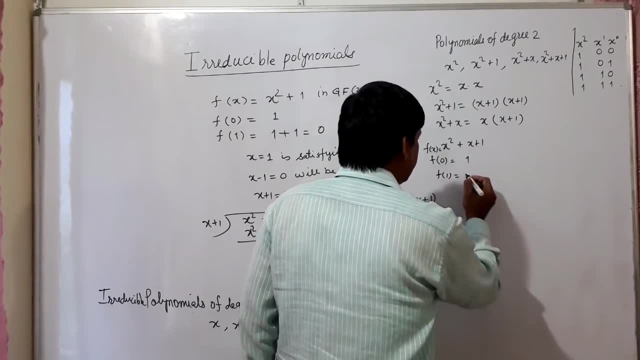 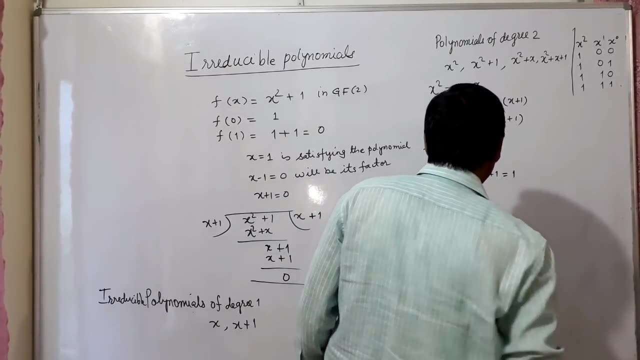 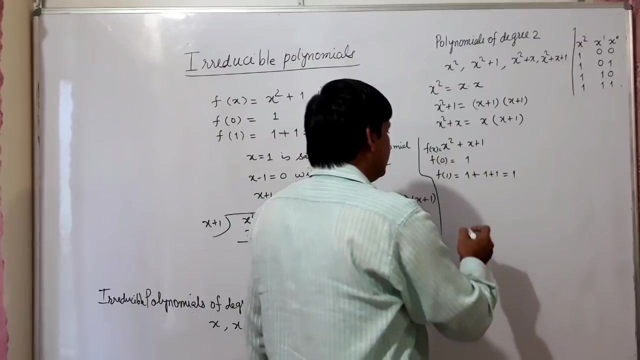 If I put 1 here, 1 into 1 is 1, plus 1 plus 1, this will come out to be 1.. So no root is there. no real root is existing here, So 1.. 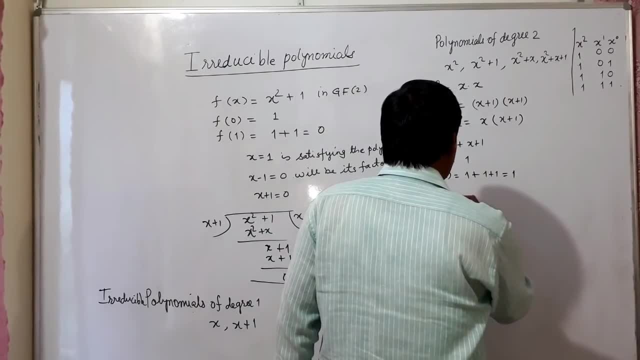 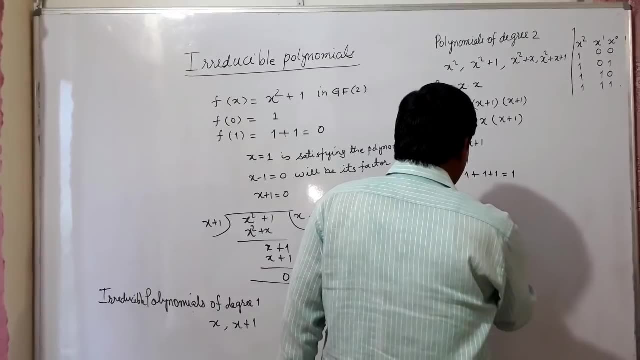 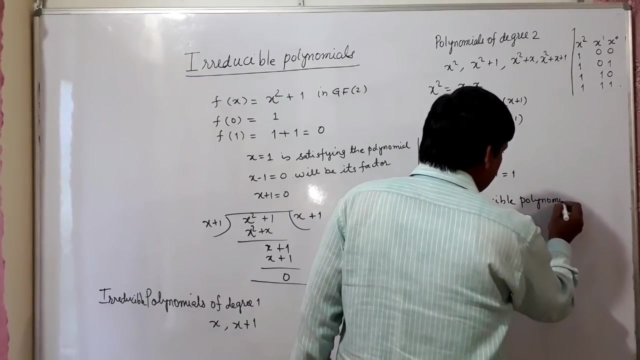 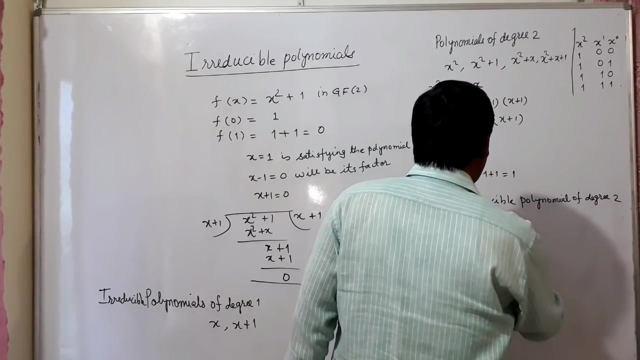 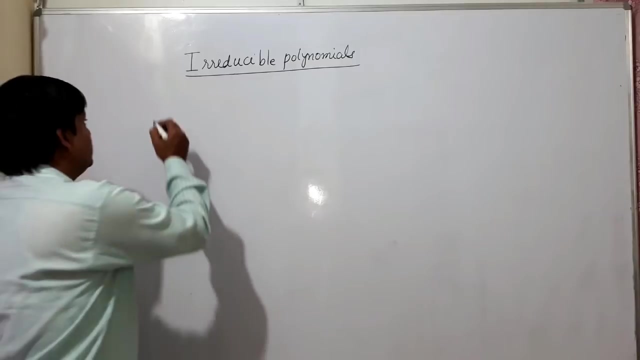 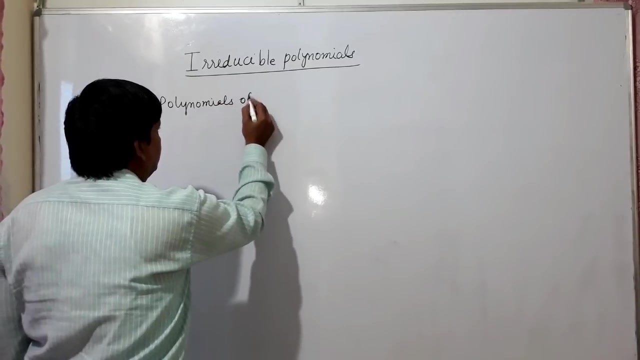 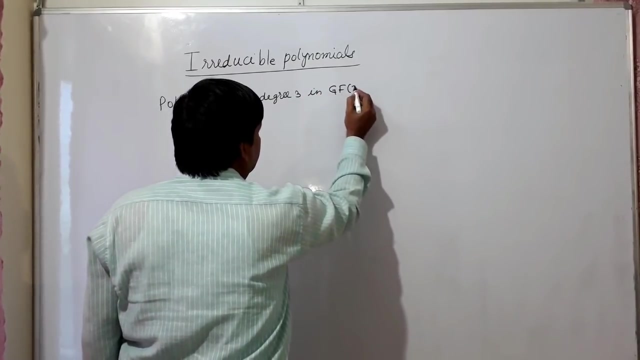 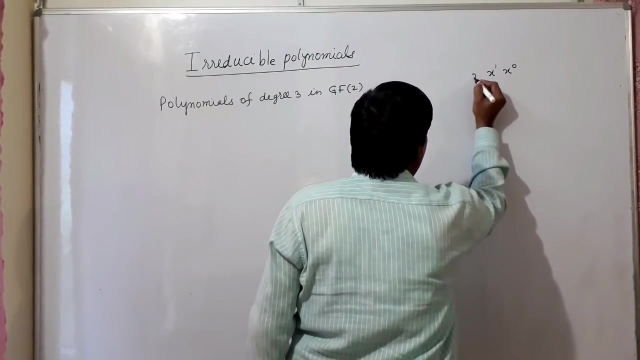 So x squared is reducible polynomial is reducible. polynomial of degree 2 will be x squared plus x plus 1.. So this is fixed. Polynomials of degree 3 in GF2, x to the power 0, x to the power 1, x squared x cube: this is fixed. 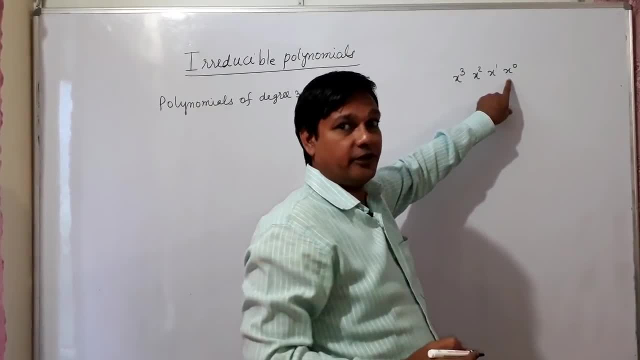 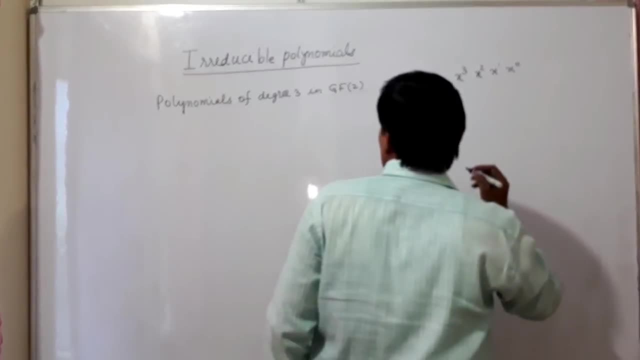 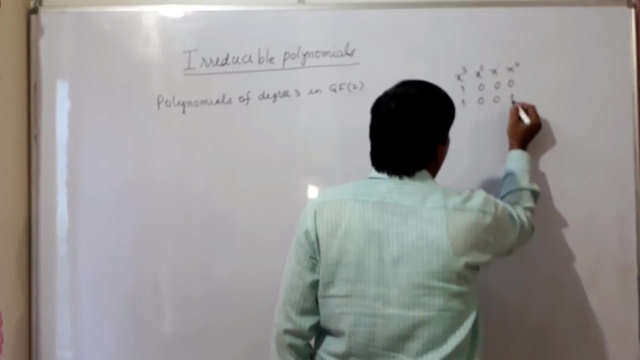 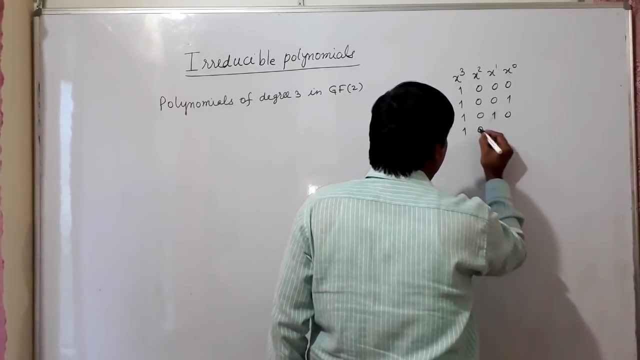 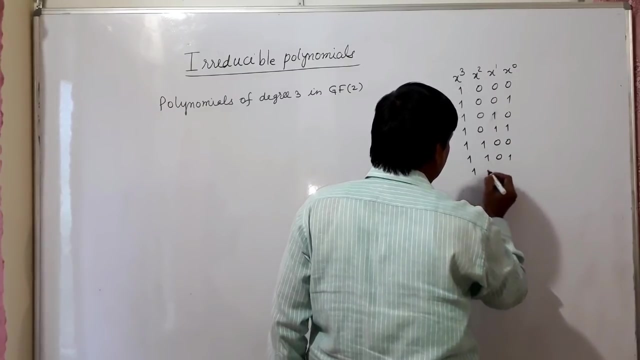 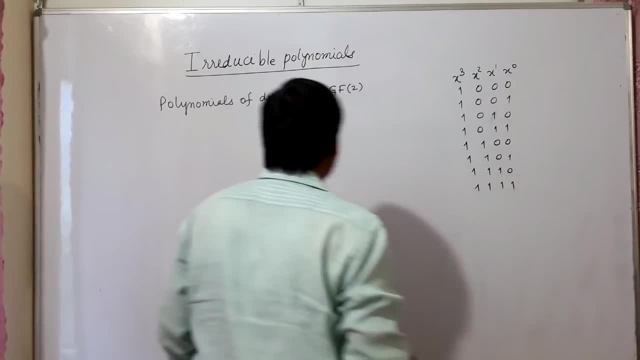 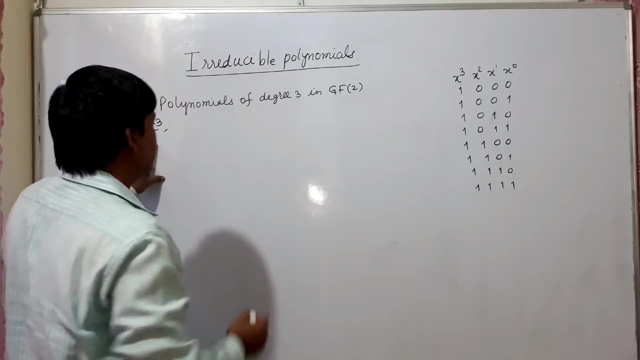 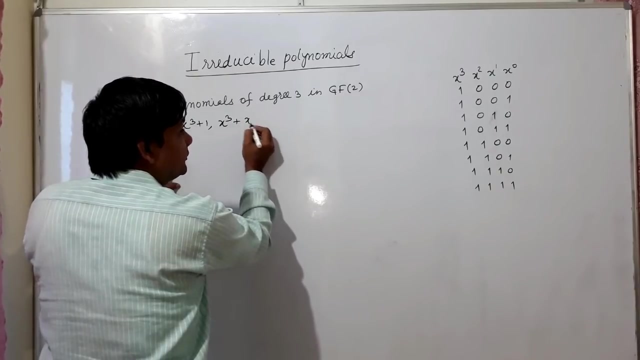 0, 1, 1, 1, 1. so you and you x cube is one polynomial of degree 3, other polynomial, x cube plus 1, x cube plus x, x cube plus x, x cube plus x plus 1.. 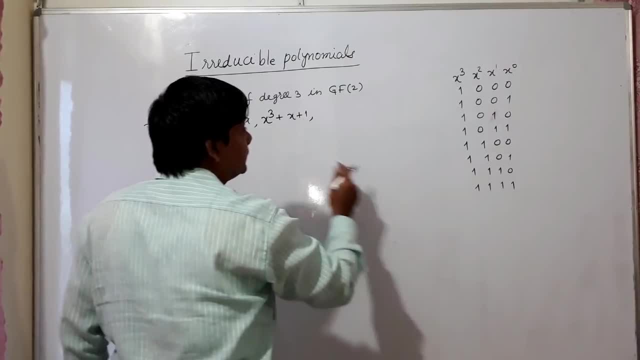 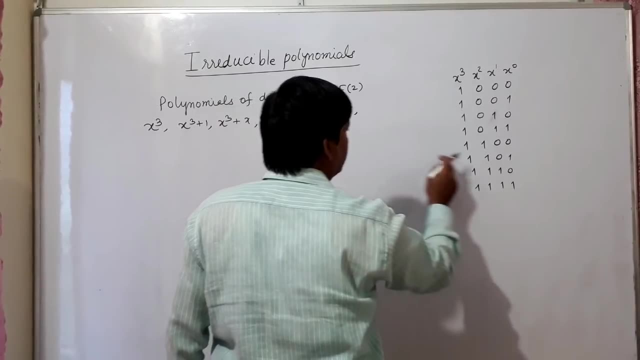 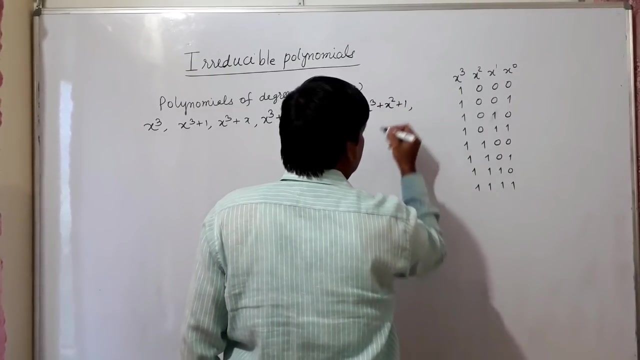 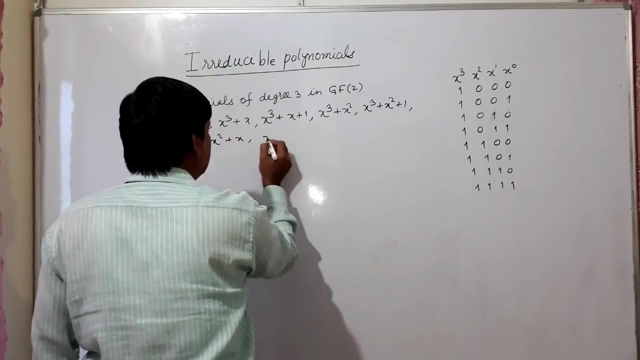 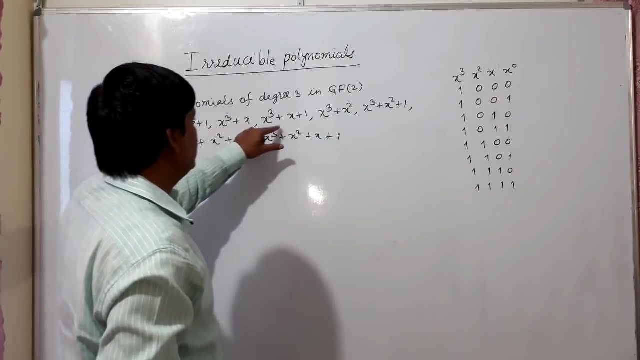 Another will be x cube plus x square. another x cube plus x square plus 1, x cube plus x square plus x. x cube plus x square plus x plus 1.. 1,, 2,, 3,, 4,, 5,, 6,, 7, 8 polynomials are there of degree 3.. 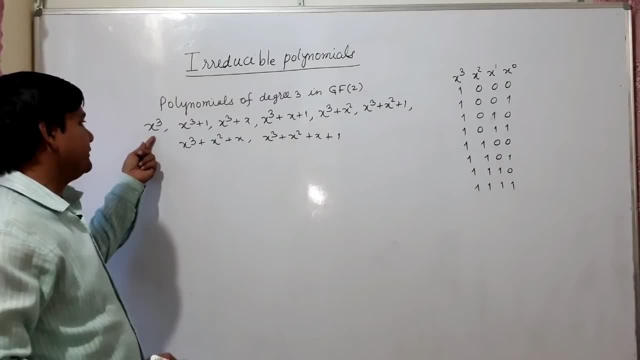 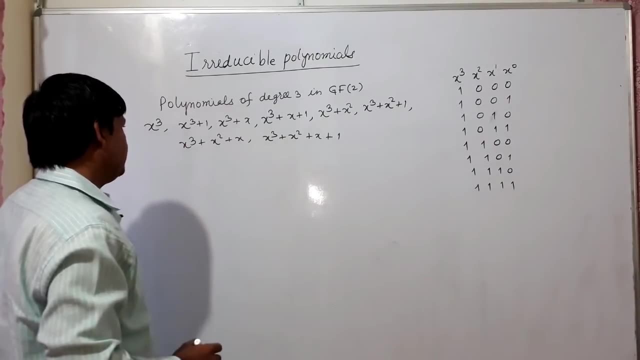 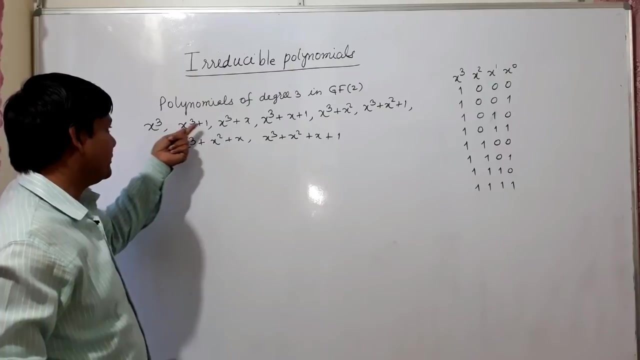 It can easily be seen: x cube can be written as x into x into x, so this is not irreducible. x cube plus 1, if I take it, if I put 1 for x, it will be 1 plus 1, 2, 2 mod 2 is 0,. 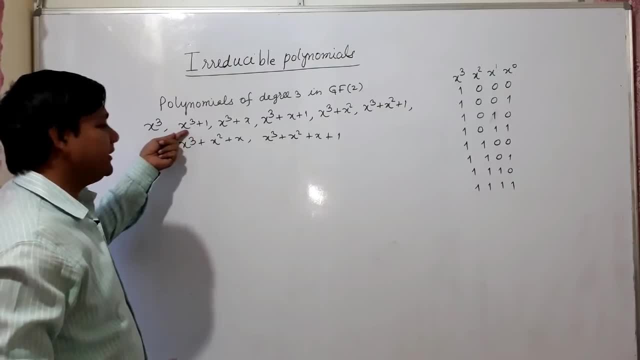 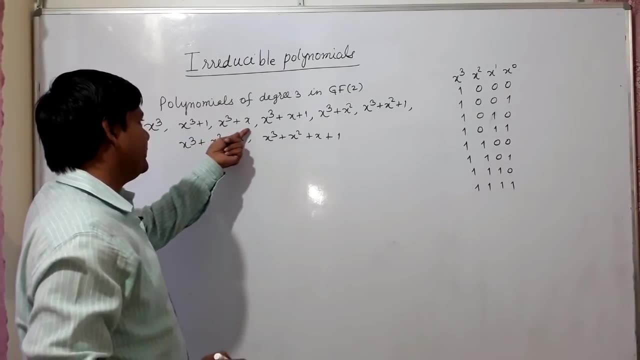 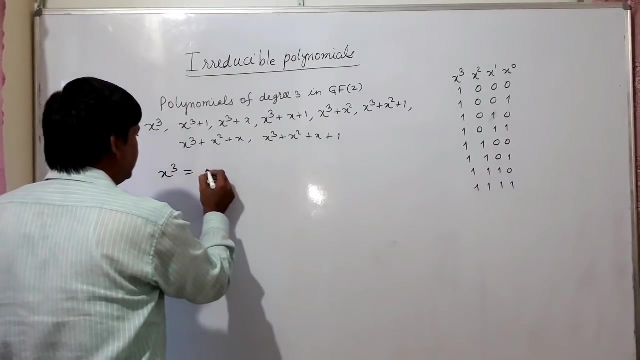 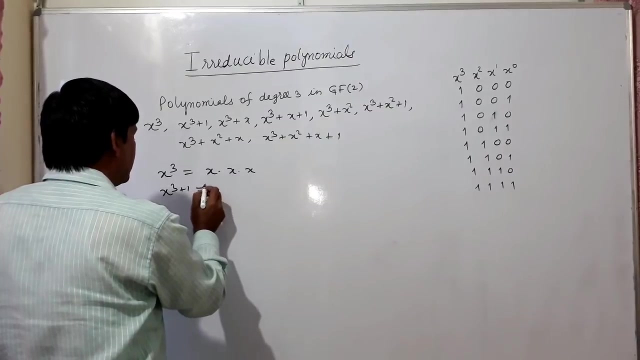 so this: This is satisfying- x equal to 1, so this is not irreducible. x cube plus x. it can be written as x into. I am writing here: x cube can be written as x into x, into x, x cube plus 1, if I take it as fx, then f1 will be. 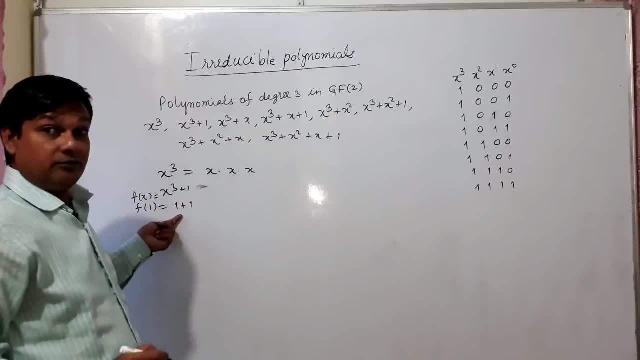 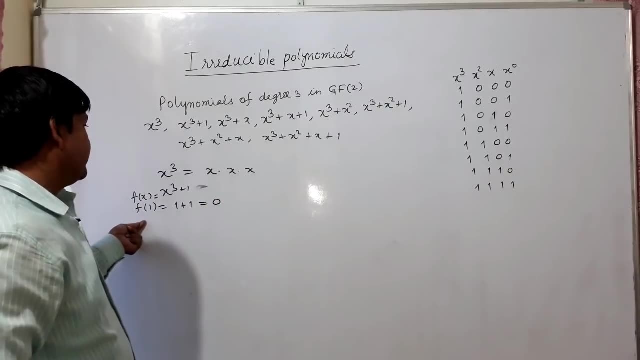 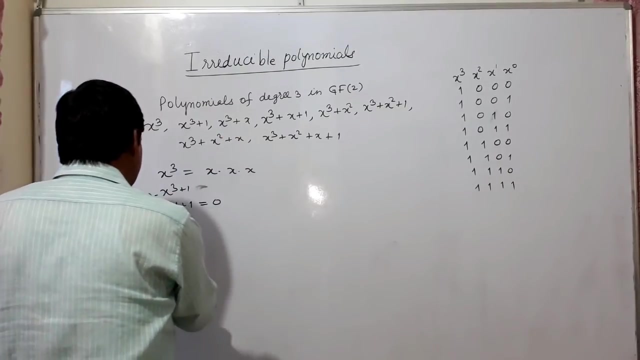 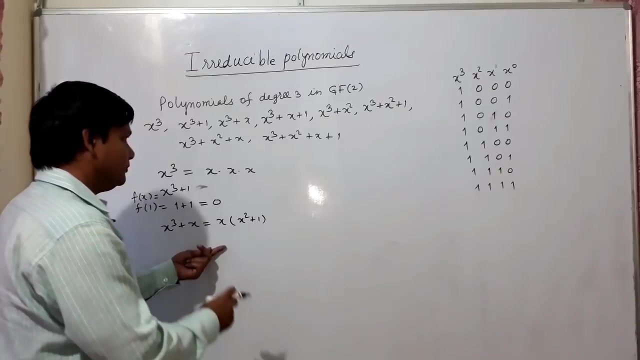 f1 plus 1,, 1 cube will be 1, and if I add 1 here, as it is it will be 0, so x minus 1 will be its root. so it is factorable. Now x cube plus x can be written as x into x square plus 1, so this can also have factors. 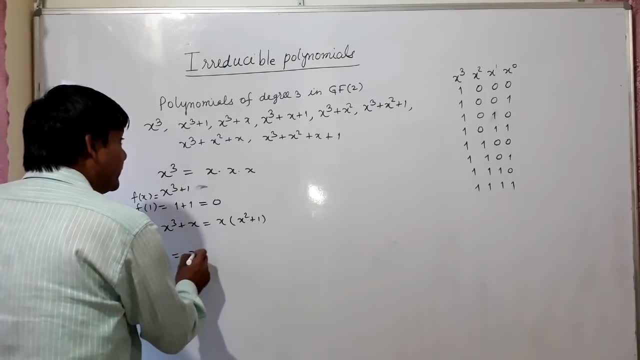 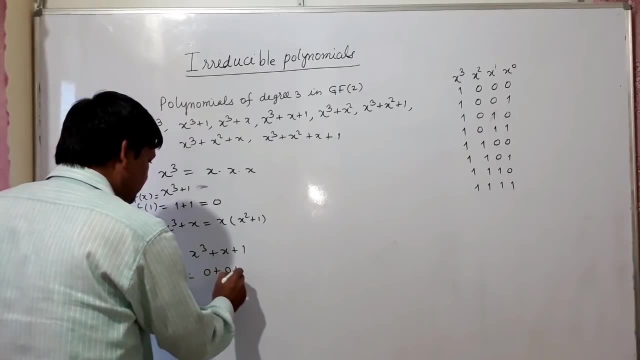 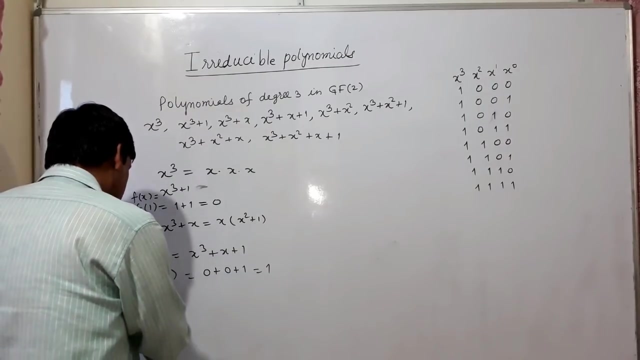 So this can also have factors. Other one is X cube plus X plus 1.. If I put 0 for X, I will get 0 plus 0 plus 1.. It will be 1.. So X equal to 0 is not its root. If I put 1 here, 1 plus 1 plus 1, which is also coming 1.. 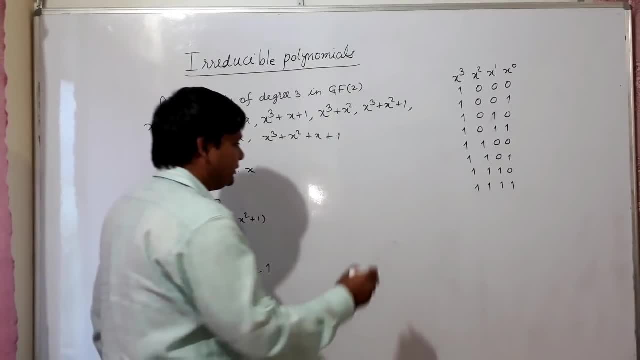 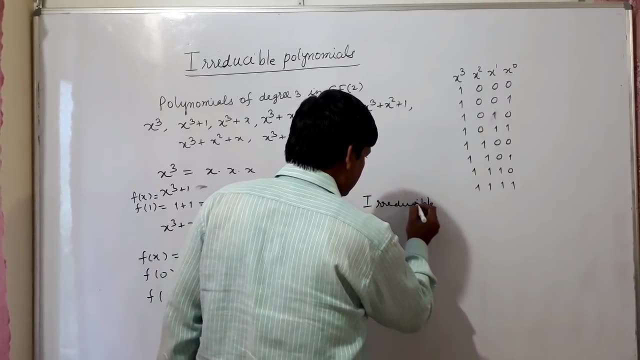 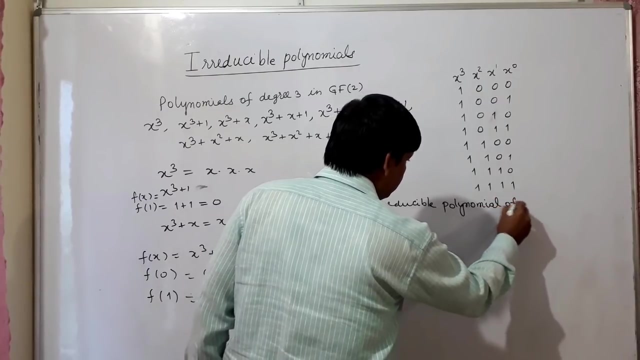 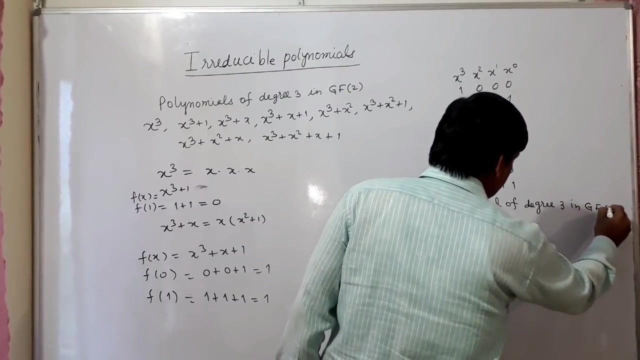 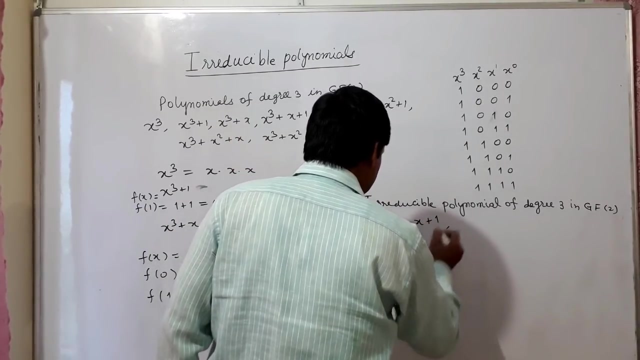 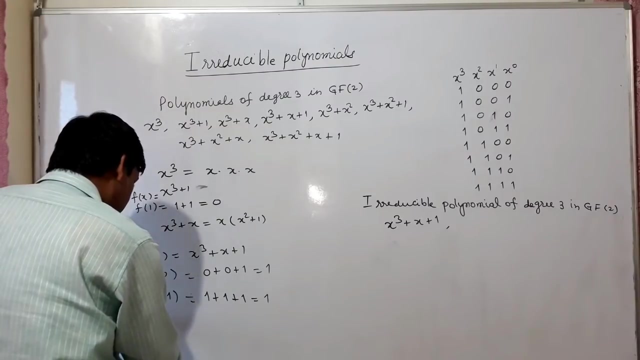 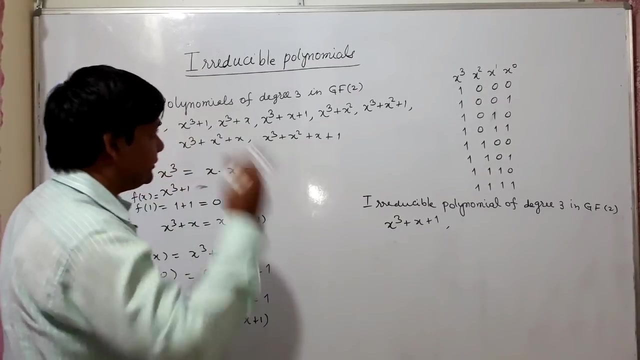 It means irredecible. polynomial of degree 3 in GF2 is X cube plus X plus 1.. We shall check some more polynomials. X cube plus X square can be written as X square into X plus 1.. So this is, it's a factor. 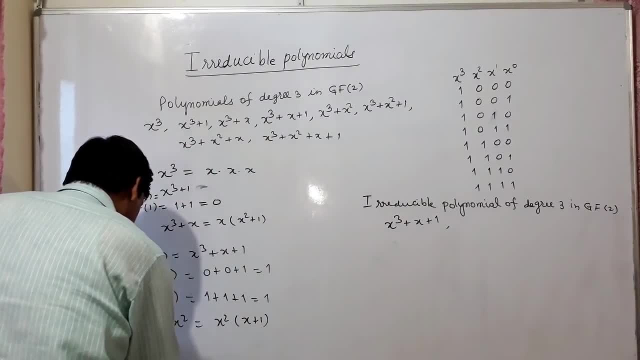 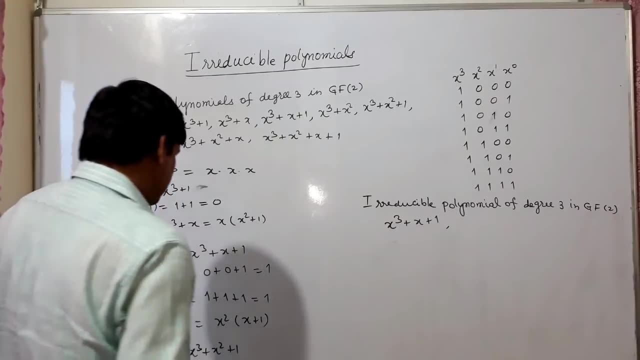 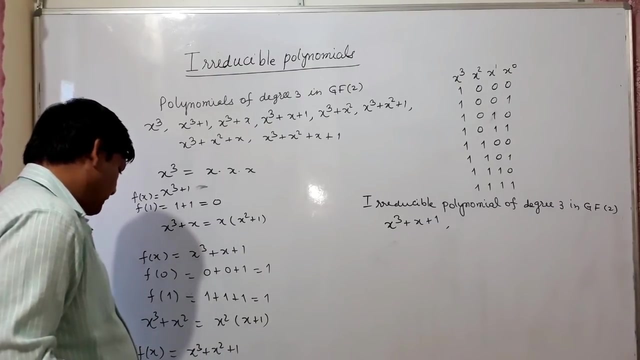 Now X cube plus X square plus 1.. If I take it as a factor, Fx, X cube plus X square plus 1.. If I put 0 for Fx, I will get 1.. And if I put 1 here, 1 plus 1 plus 1, which will also be 1.. 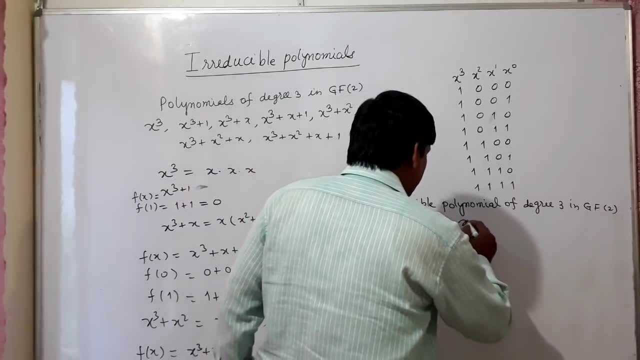 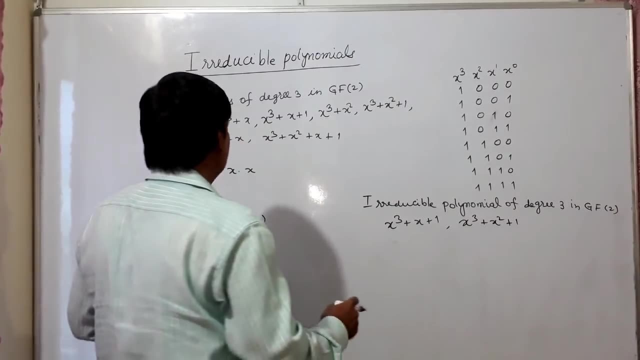 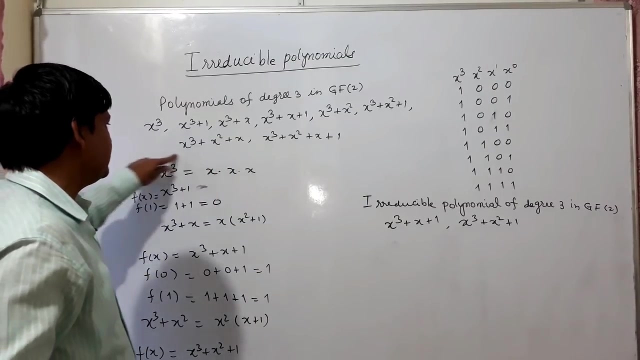 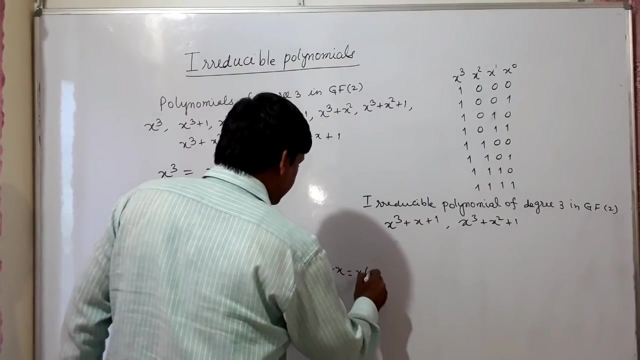 So this is irredecible: X cube plus X square plus 1.. And X cube plus X square plus X X, is its a factor? Clearly it is. We can see here: X cube plus X square plus X X into X square plus X plus 1.. 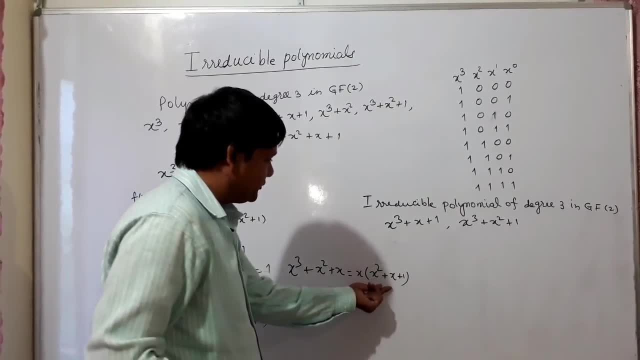 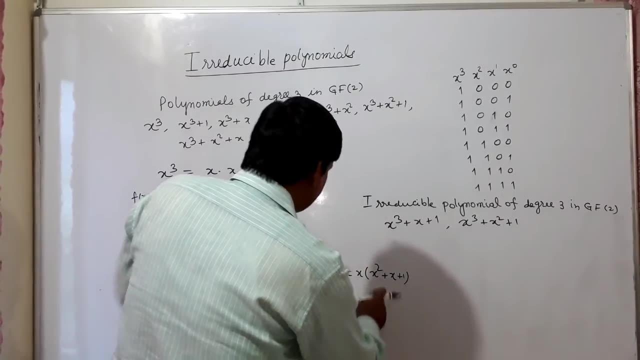 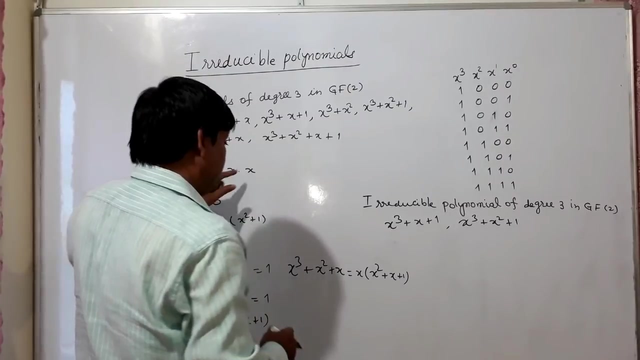 So these are the factors. I am not checking their factors, I am not checking factor of this polynomial, But it's irredecible. We have already seen in degree 2.. So no problem, But it's, We are getting these two factors here. 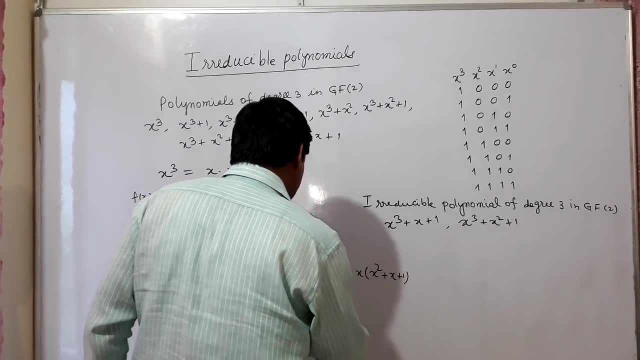 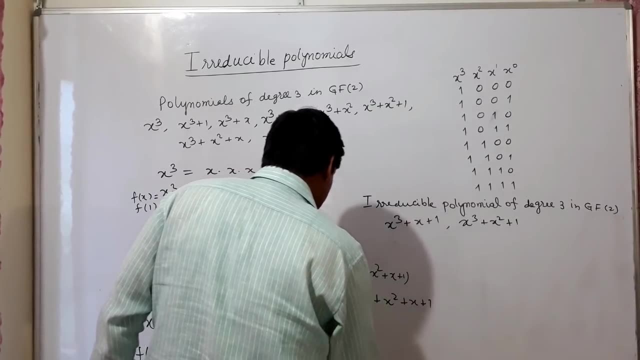 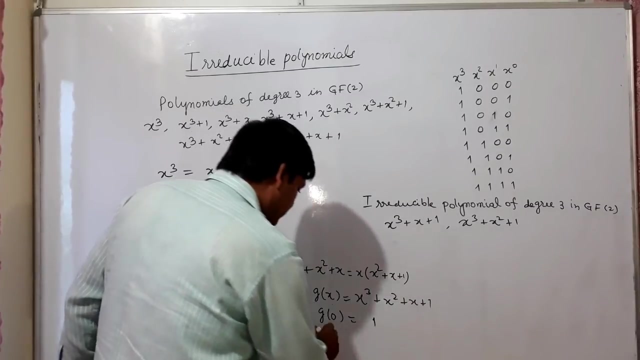 And one more polynomial is there. If I take it, ZX is equal to X cube plus X square plus X plus 1.. If I put 0 here, we are getting 1.. 0 plus 0 plus 0 plus 1, 1.. 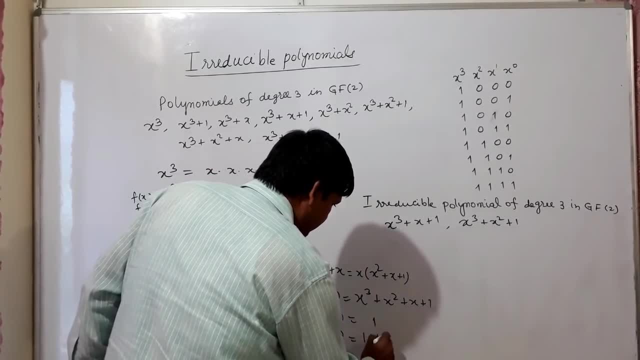 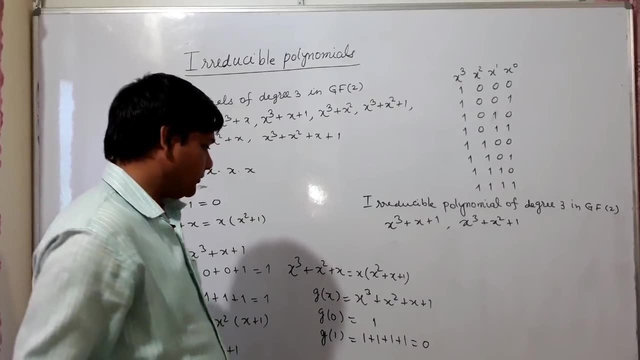 If I put 1 here, we are getting 1 plus 1 plus 1 plus 1, which is coming 0.. X minus 1 will be its root. X minus 1 will be its factor. X equal to 1 will be its root. 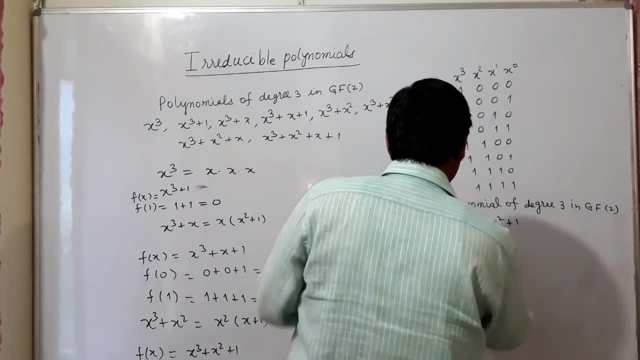 So irredecible polynomial of degree 3 in GF2 will be these two only.